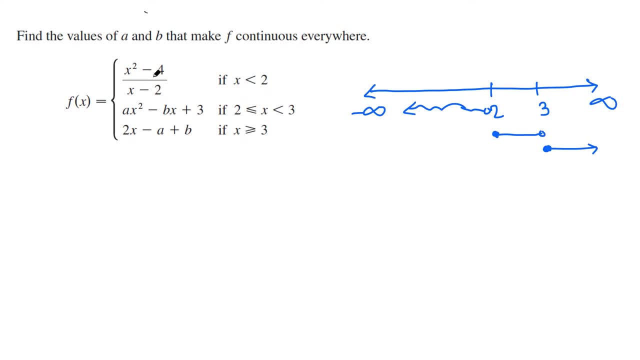 So each piece is continuous. so the issue here is at the endpoints: what happens at 2 and 3?? If this function is continuous at 2 and 3, then this will be continuous everywhere. so the issue here: there are two places are at. x equals 2 and 3. 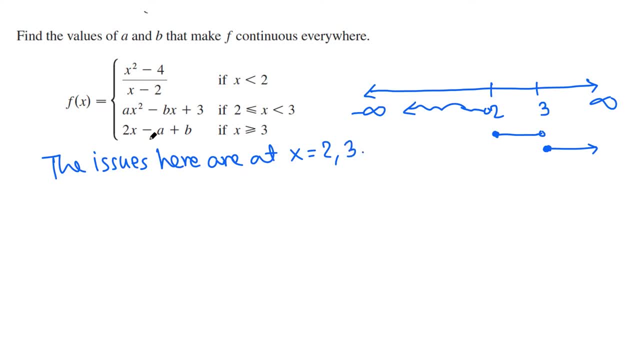 and for a function to be continuous, I mean we need to satisfy three cases at least. the limit at that values- x values- should exist. limit exist means left hand, limit should be equal to right hand. So I'm going to apply that. so for f, for the limit of f, it to exist, means limit of the function. 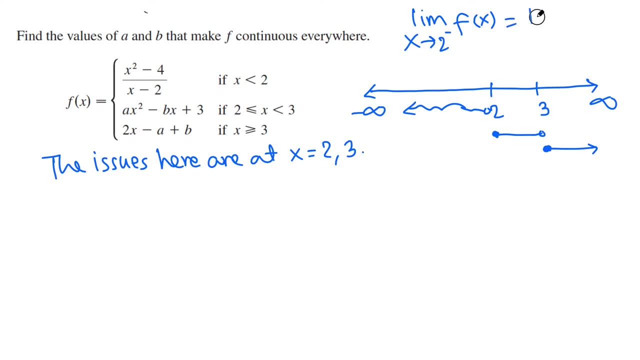 when x approaches to 2 from left should be equal to limit of the function. when x approaches to 2 from right, this should be the same, so that limit exists and we have more conditions to satisfy. but this is necessary condition and same thing at 3.. 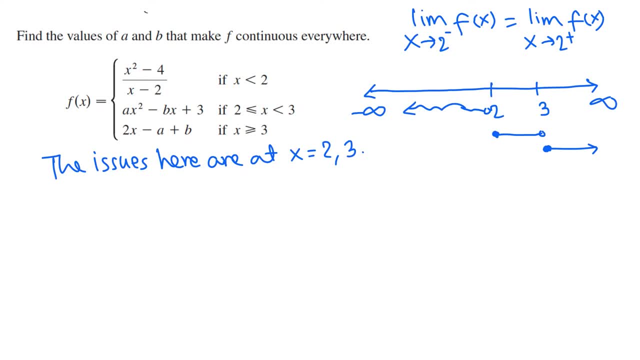 So at 2 for left hand limit, I mean the left. so that's the left part and this is the right part. so for 2, this will be the left and this will be the right. so I'm going to find the limits there, okay. so 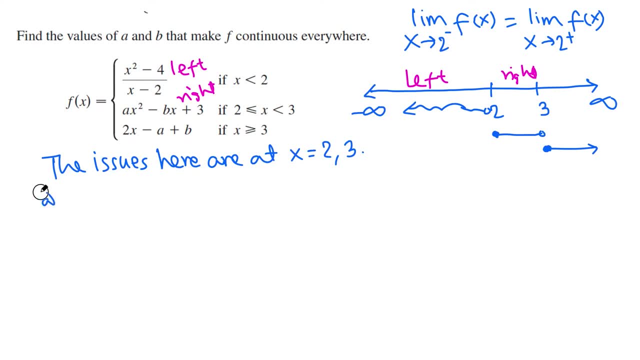 at 2 limit of the function when x approaches to 2 from left, is limit? x approaches to 2 from left of this function. this piece x square minus 4 over x minus 2.. Now this negative is nothing, just for the limit. if we directly plug in, x equals 2, 2 square 4 minus 4, 0 over 0. 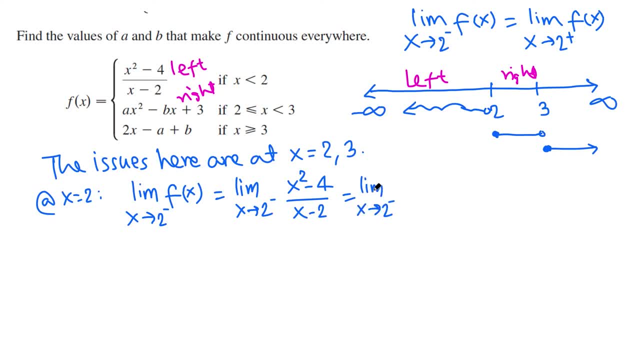 so we need to simplify before we plug in. simplify means factor the top. this is a difference of 2 squares. so we get x plus 2, x minus 2 on the bottom. we already have x minus 2. cancel. now plug in 2. this negative is just for the direction: 2 plus 2- 4.. 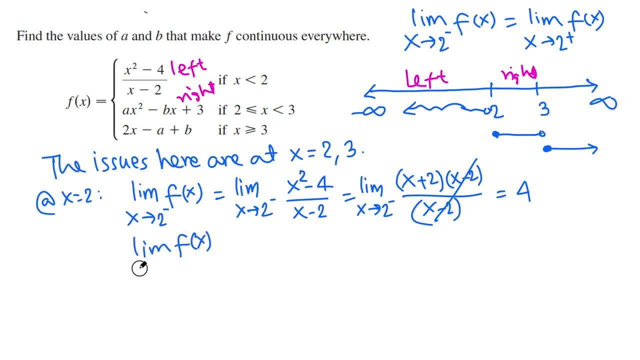 Now, similarly, we want to find the right hand limit when x approaches to 2 from right side- right side. so we're going to use this polynomial. so limit x going to 2 from right side of ax squared minus bx plus 3: oh, this is a polynomial, so all we have to do is simply plug in. 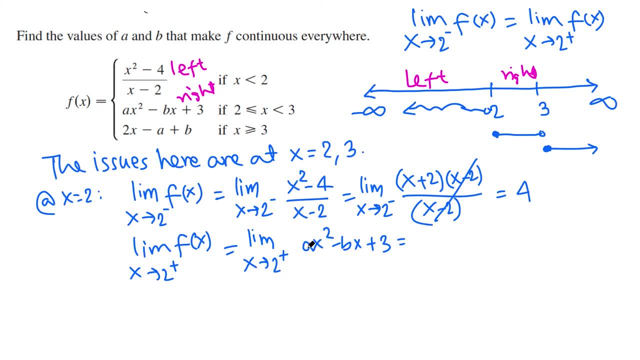 2 for x. so 2 is squared 4a minus b times 2, 2b plus 3. so this is left hand limit at 2 and this is right hand limit at 2.. For the function to be continuous at 2, left hand limit should equal right hand limit. 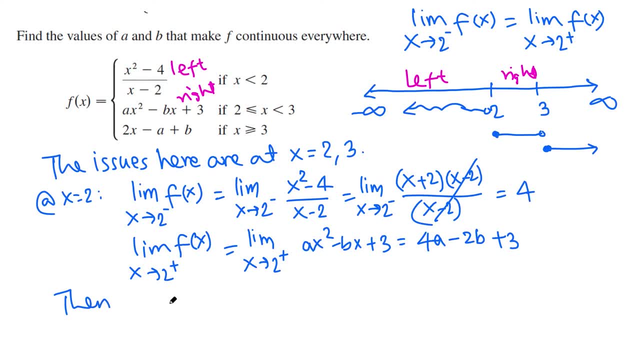 then this right hand limit. let me write this first: 4a minus 2b plus 3 should equal 4.. From this we cannot determine a and b, because only one equation. but let me subtract 3 from both sides and I get a nice equation: 4a minus 2b equals 1,. 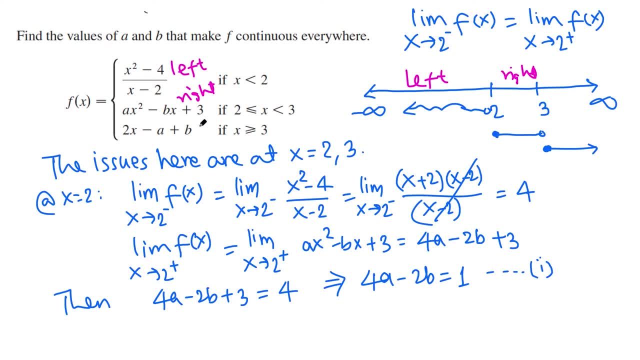 for future reference, I'm going to write: 1. Now we do the same type of work at 3, so when we are considering at 3, okay for 3, this function will be left and this one will be right. so this is left and the function is right, okay. 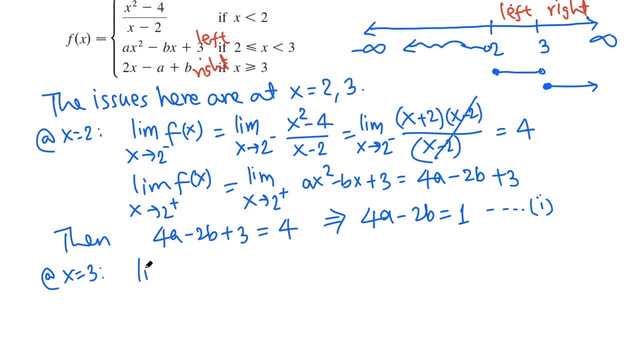 at 3 limit of f when x approaches to 3 from left, is limit x approaches 3 from left. so this: a x squared minus bx plus 3.. This is a polynomial, so all we have to do is just plug in: x equals 3,. 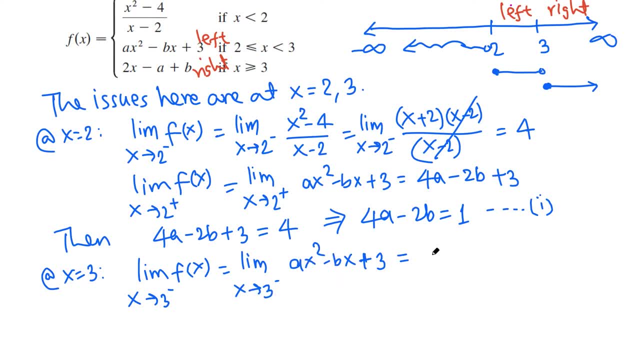 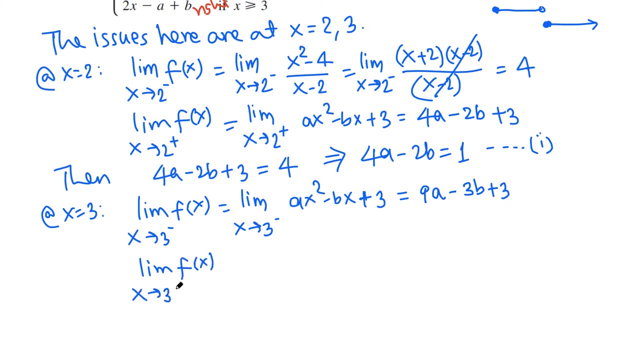 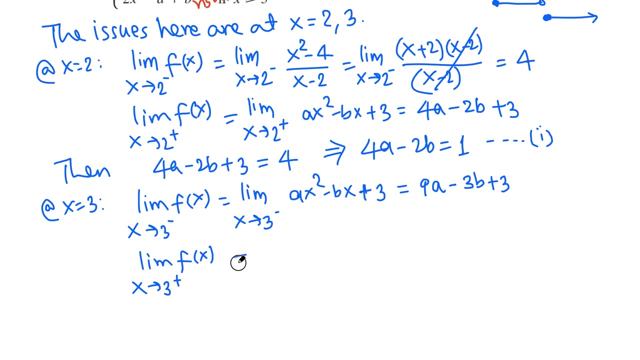 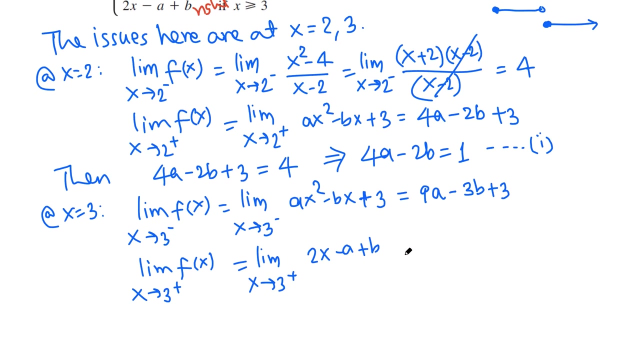 3 squared: 9a minus 3b plus 3. okay, Now let me find right hand limit when x approaches to 3. so the very last function: 2x minus a plus b. This is a polynomial, so all we have to do is simply plug in x. 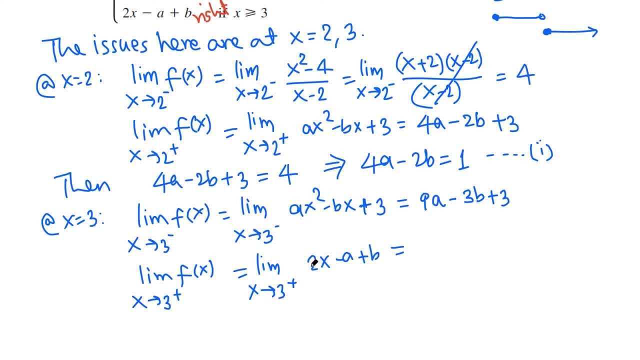 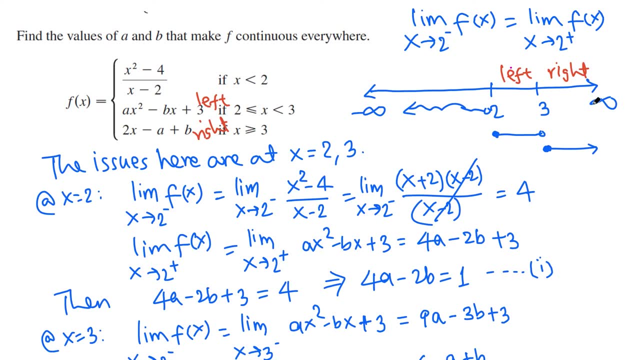 so all we have to do is simply plug in. x equals 3, so 3 2 times 3 is 6 minus a plus b, and for the function to be continuous everywhere, it has to be continuous at 3. that means this should be same. 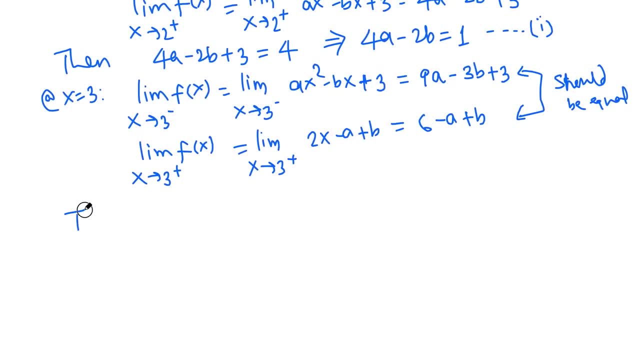 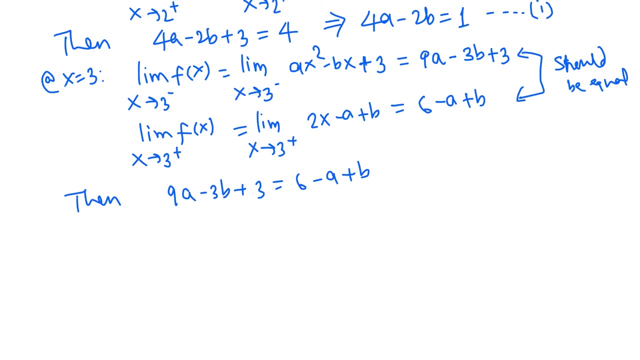 okay, that means 9a minus 3b plus 3 is 3.. 9a minus 3b plus 3 is t. 3b plus 3 is 6 minus a plus b. Let me write a nice function, so I want to bring. 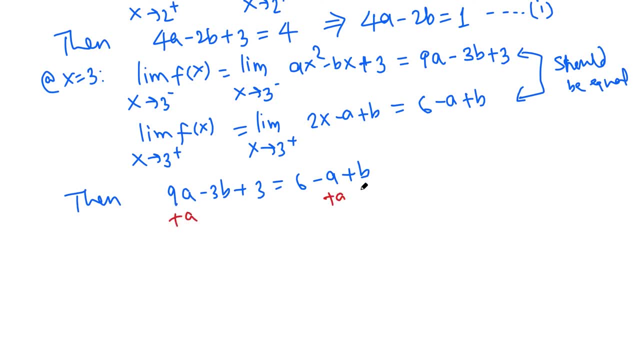 a to the left side. so add a subtract b and subtract 3 to move number over. that gives 9 a plus a, 10 a minus 3b minus b minus 4b equals 3. so we cannot find a and b because we have only one equation and two unknowns. so I can call this: 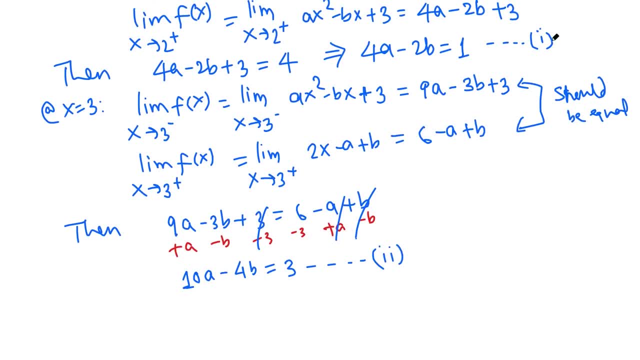 equation 2.. Now we have equation 1 on variables a and b, and same thing here. Now we got a system of linear equations and we know how to solve using college algebra, so we can use method of elimination or method of substitution or graphing. So let me put them together. this is equation 2. I'm 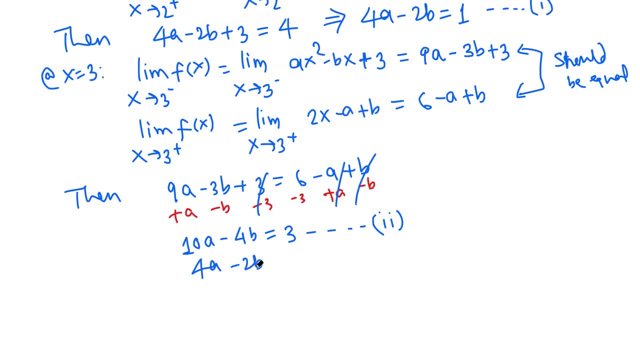 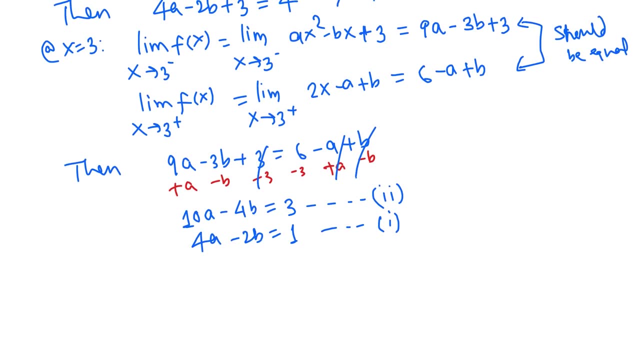 gonna write equation 1 together: 4a minus 2b equals 1, looking at this, 4b- 2b, I want to use the method of elimination. I want to multiply equation 2 by negative 2 so that this becomes negative minus negative, positive. 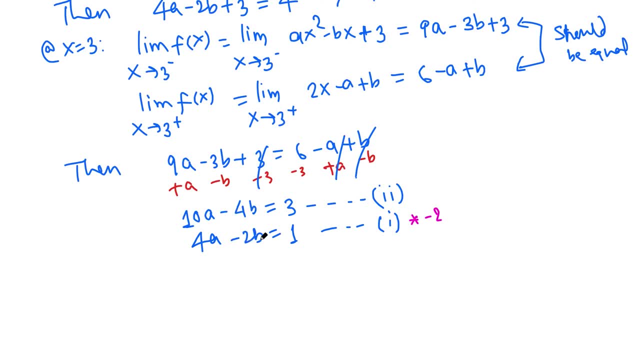 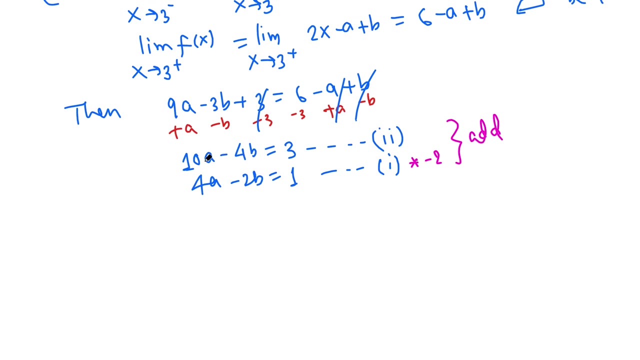 4b, and when I add negative 4b plus 4b will be 0. so I can eliminate variable b, then I can determine the value of a. So I want to multiply by negative 2, then add these two equations. okay. So I didn't do anything for equation 2, so this is 10a. 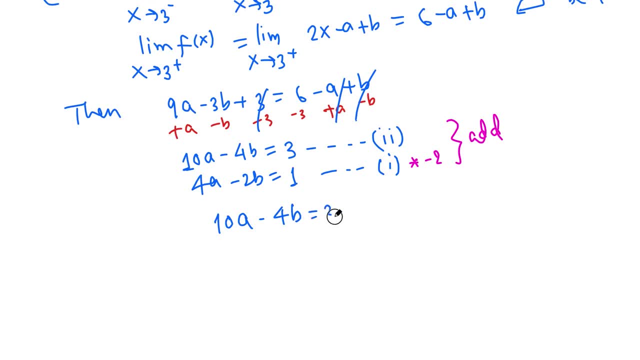 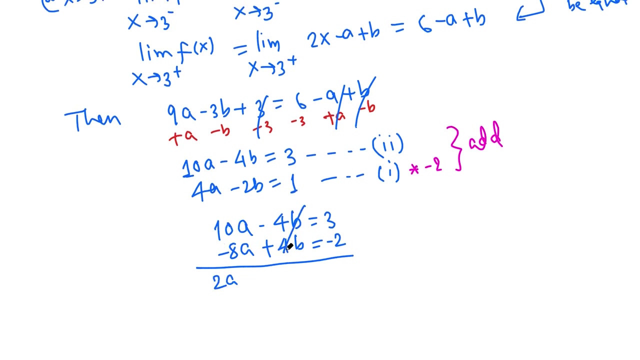 minus 4b equals 3, multiplying by negative 2, negative 8a plus 4b equals negative 2. so we are adding that means 10a minus 8a, 2a- cancel. that was the purpose and that equals 1. so this implies a equals 1 half. so we found the